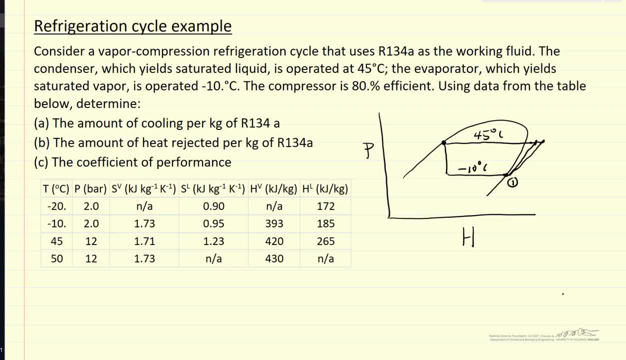 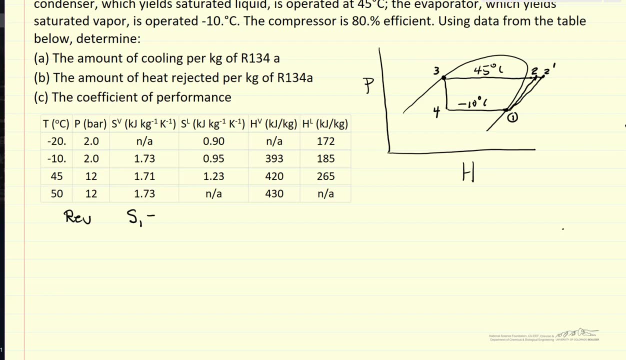 and let me label these points one, and i'll call this point two reversible, and then the actual, the irreversible, let's call it two prime, three and four. so first calculation. then is the compressor for the reversible case: s1, 1, 1, S2 and s1. this is saturated vapor minus 10 degrees c. so saturated vapor minus 10 degrees c. here's the. 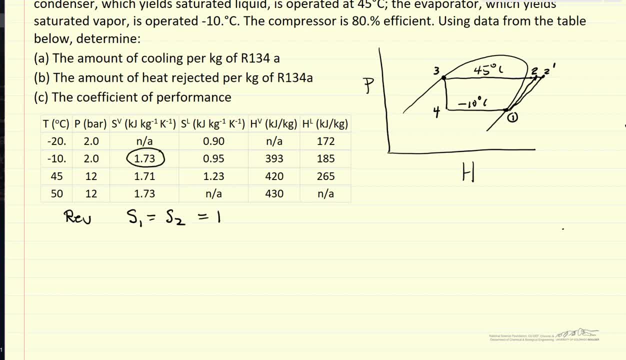 entropy. so s1, which is equal to s2, is 1.73 kilojoules per kilogram degrees kelvin. so s2 now has to have that same entropy because s2 is at a higher pressure. well, the pressure is 12 bar, because we can see. 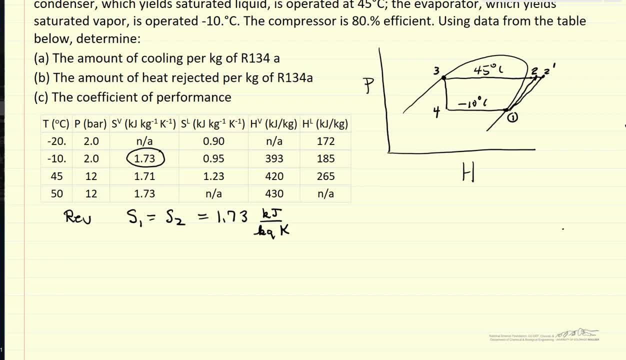 here the 12 bar. that that's for the case where we have liquid and vapor. so 45 degrees is the saturation temperature. we're at a higher temperature but the same pressure. so here is the value corresponding to our condition s2. so this means we know the enthalpy at two and that's 430 kilojoules per kilogram. well, enthalpy at one, the saturated vapor minus 10 degrees is 393.. 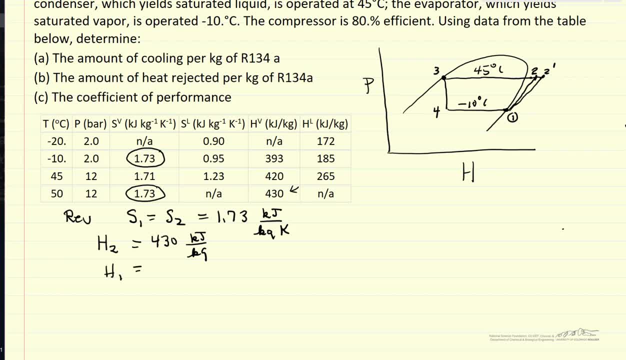 1, the saturated vapor minus 10 degrees is 393.. 1, the saturated vapor minus 10 degrees is 393.. 2, the saturated vapor minus 10 degrees is 393.. And so we can calculate delta H then for the reversible compressor, and that's H2 minus H1,. 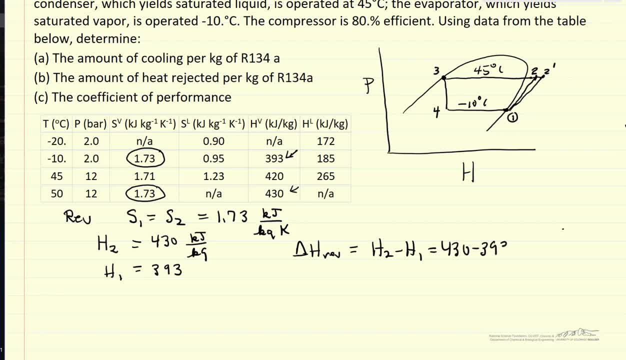 so that's 430 minus 393, and that's 37 kilojoules per kilogram. So remember, this is reversible. The delta H is equal to the work. so the work reversible is delta H reversible because it's adiabatic. so we know the work we have to add for the reversible case. Well, what we're? 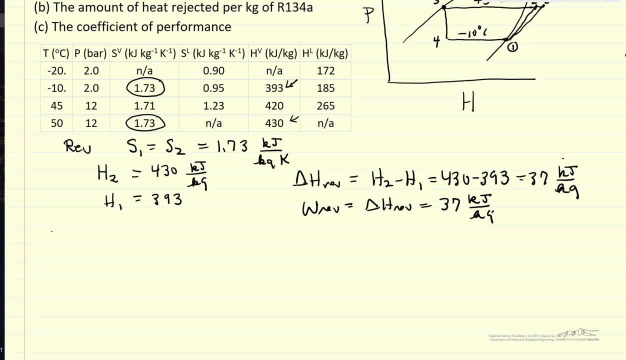 interested in is the irreversible case. so the work for the irreversible case, when the efficiency is 0.8, the work has to be more so it's the reversible work: over 0.8, 37, over 0.8, 40,. 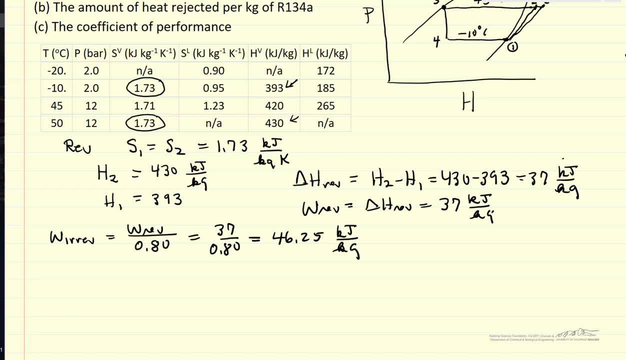 let's keep the significant figures for now. The work is larger. this is the irreversible work. Well, the irreversible work, then, is the enthalpy change for the irreversible. so that's H2 prime minus H1.. Which means H2 prime is H1 plus 46.25.. Well, we already used H1, already right. H1, 393 kilojoules. 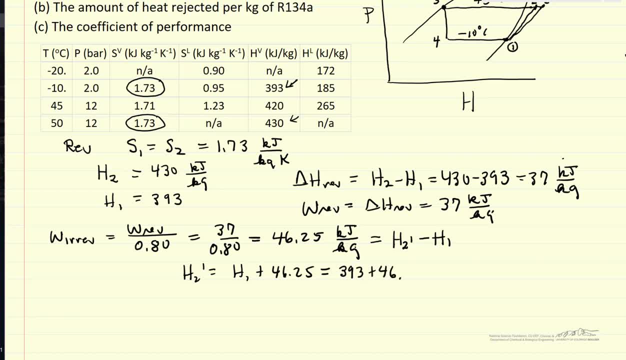 per kilogram. 393 plus 46.25, so 439 kilojoules per kilogram is the enthalpy at 2.. Now calculate the heat. We need enthalpy at 3.. Enthalpy at 3 is saturated. 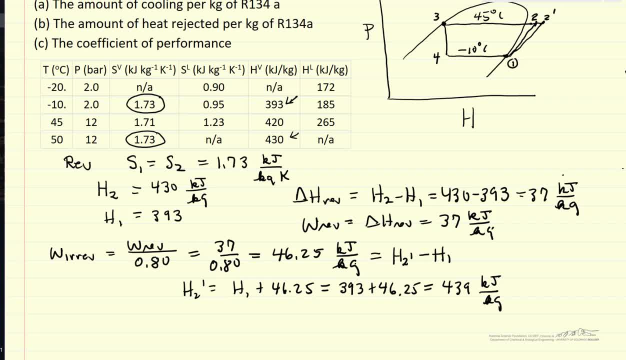 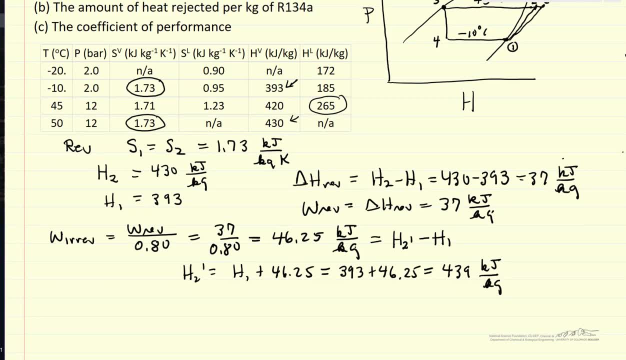 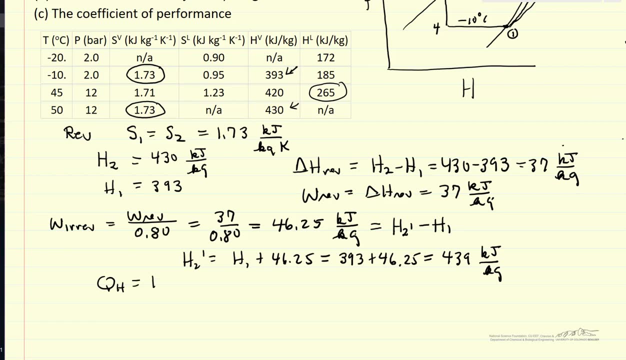 Liquid 45 degrees C. so 45 degrees saturated liquid. Here's the enthalpy. So the change as we condense this fluid, condense it by removing energy, so heat that we remove, that's at the high temperature, would be H3 minus H2 prime. 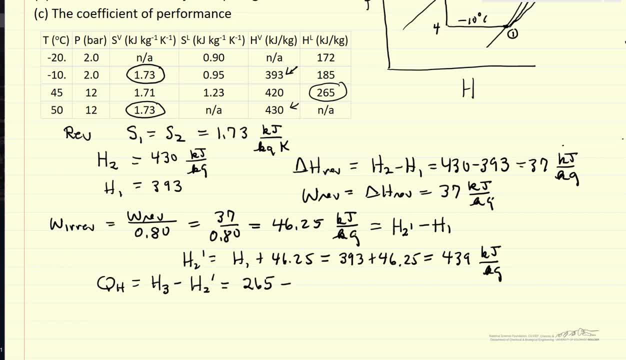 Sol at 265 is the saturated liquid, and we just calculate it. That 439 was the entering into that condenser, So QH then minus 174 kilojoules per kilogram. Well, this is one of the values we wanted to calculate for the problem statement. So, finished one part and we're going. 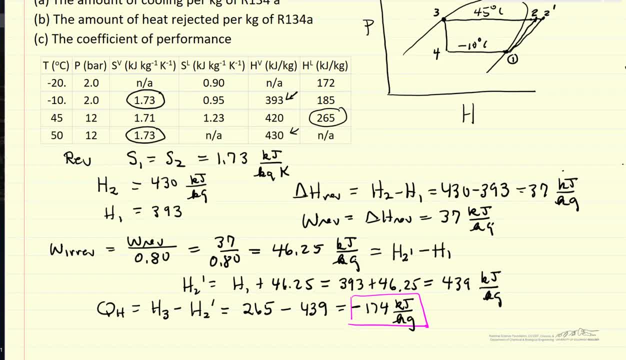 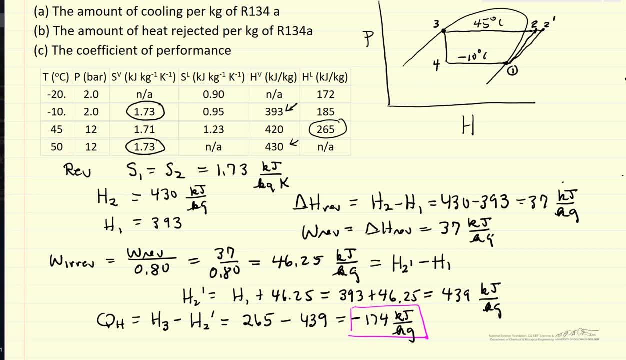 to now calculate QC. So, keeping in mind the diagram, we're going to need H4, but H4 is the same as H3 because we're going through a throttle. So H4 then is our 265. So this is also 265 kilojoules per kilogram, And H1- we've already calculated 393.. So that means, if we want to, 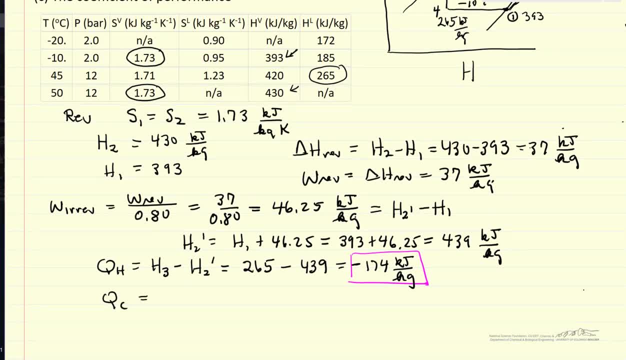 calculate QC. this is the cooling. how much energy we remove from our low temperature refrigeration section of a refrigerator put in at minus 10 degrees into this cycle? that's the cooling, So that's the cooling. So that's the cooling, So that's the cooling. 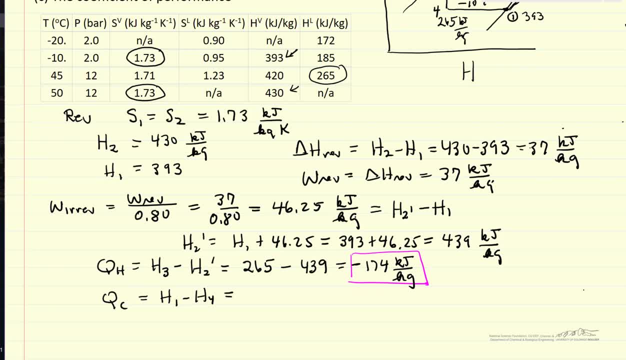 That's H1 minus H4, the final minus initial, And H1 is 393.. H4, 265.. So this is 128.. And it's positive because we're adding energy into our cycle. So this is QC. Remember, this is QH.